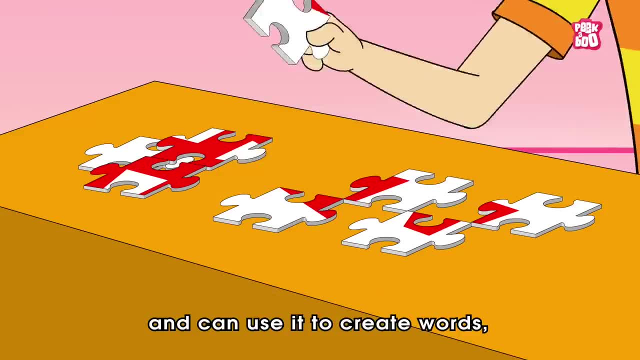 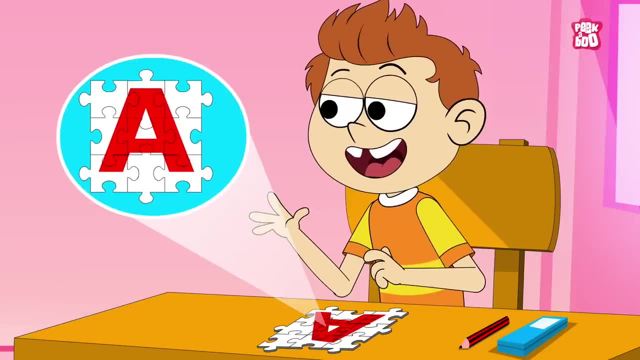 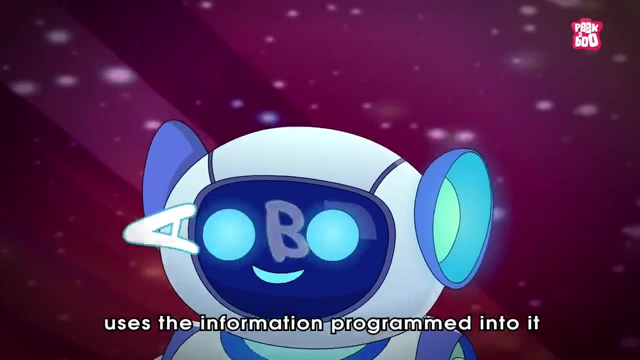 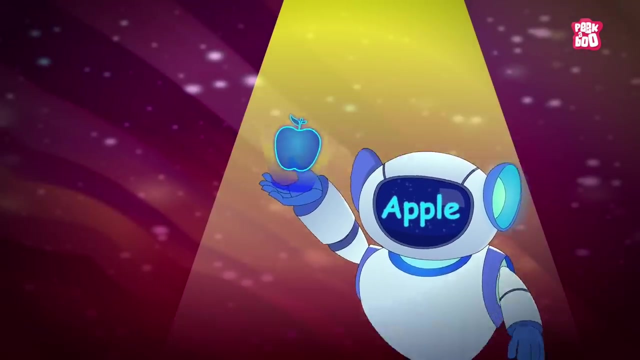 we acquire this information and can use it to create words, sentences or even solve many problems. Similarly, when a robot or computer uses the information programmed into it to solve problems, it is also using a form of intelligence. However, this type of intelligence is different from human intelligence. 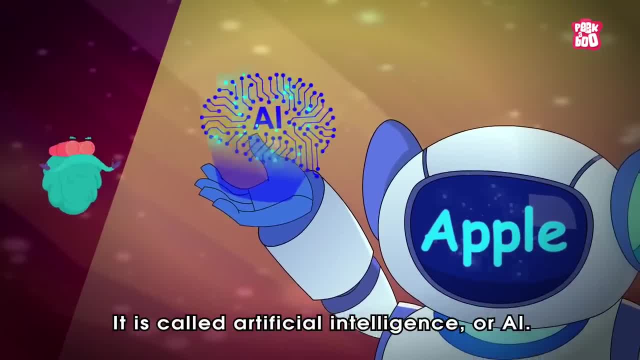 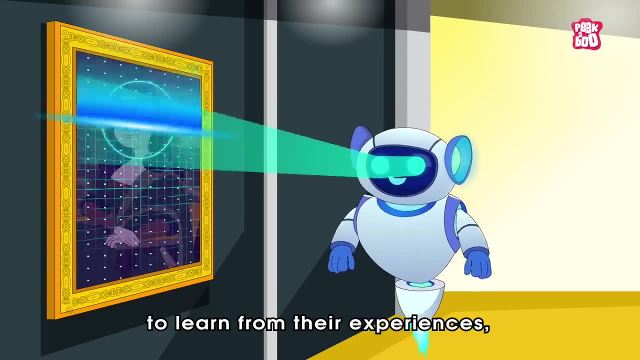 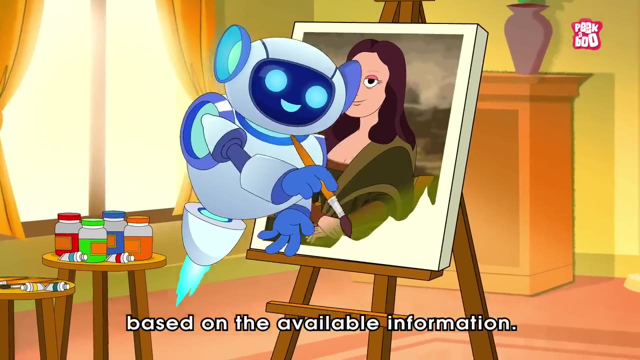 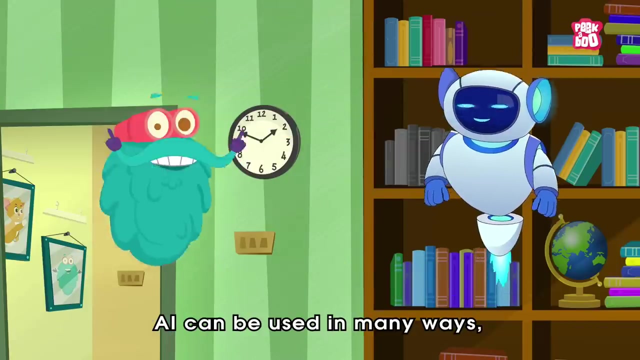 It is called artificial intelligence or AI. AI systems are designed to be able to learn from their experiences, adapt to new situations and make decisions based on the available information. But the crucial question is: is it really helpful to us? AI can be used in many ways, from helping humans perform tasks more efficiently. 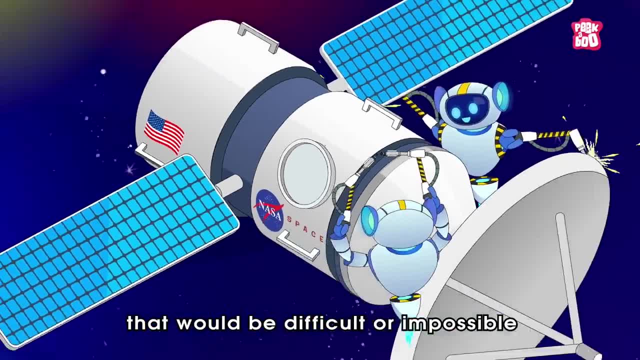 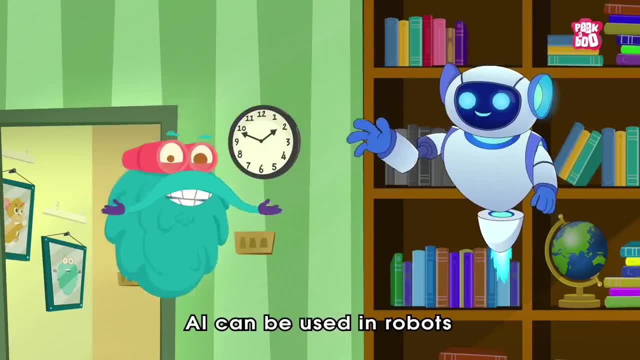 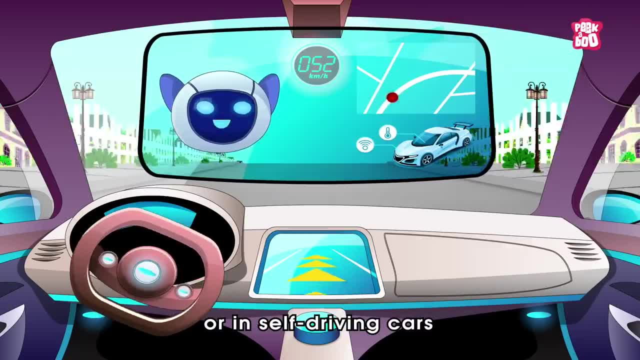 AI can be used in robots to help them do tasks in factories, or in self-driving cars to help them navigate roads and avoid accidents. AI can be used in robots to help them do tasks in factories or in self-driving cars to help them navigate roads and avoid accidents. 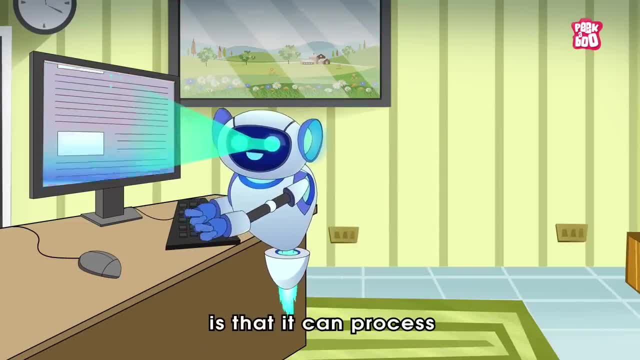 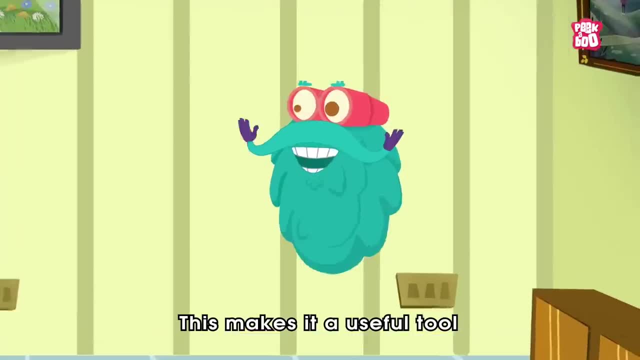 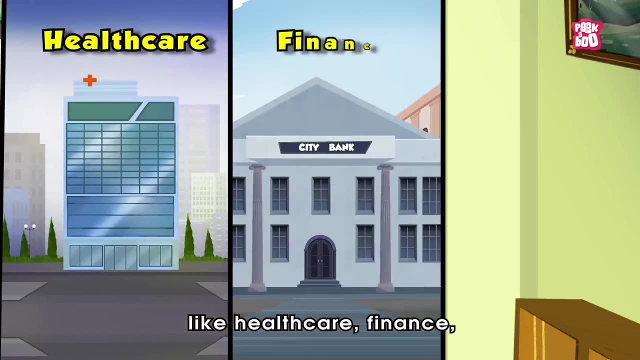 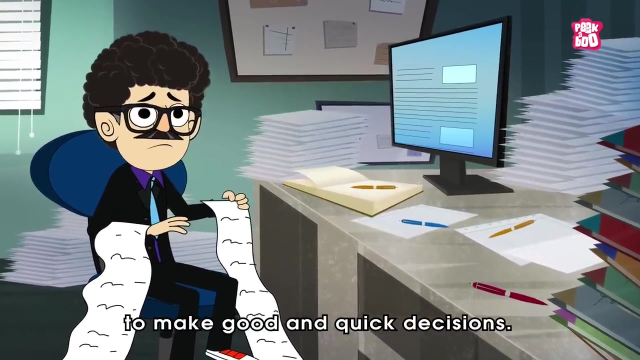 One of the best things about AI is that it can process and analyze- although problems or errors- lots of data very quickly and accurately. This makes it a useful tool in many different industries like health care, finance and retail. lots of data needs to be analyzed to make good and quick decisions, so in a way, it is a very powerful 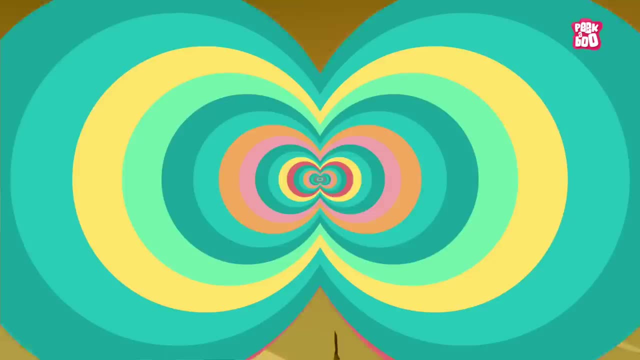 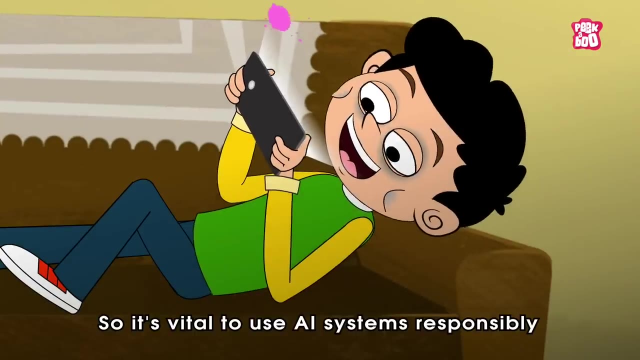 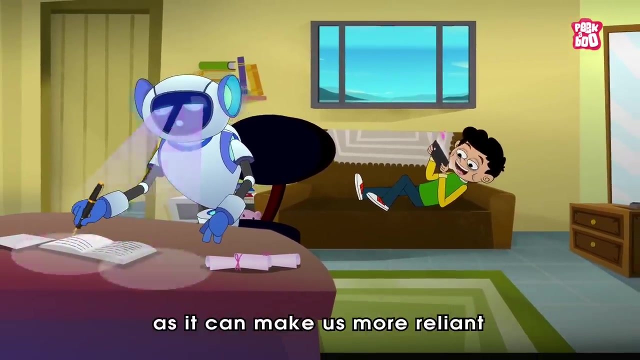 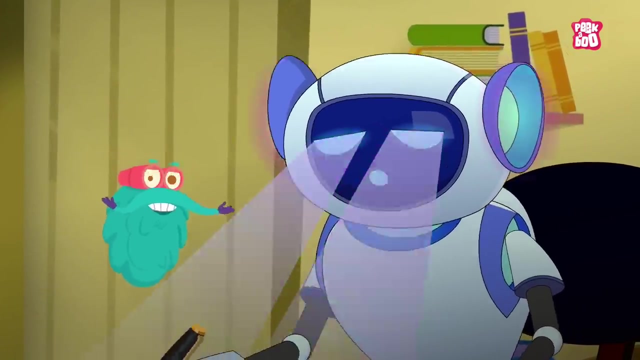 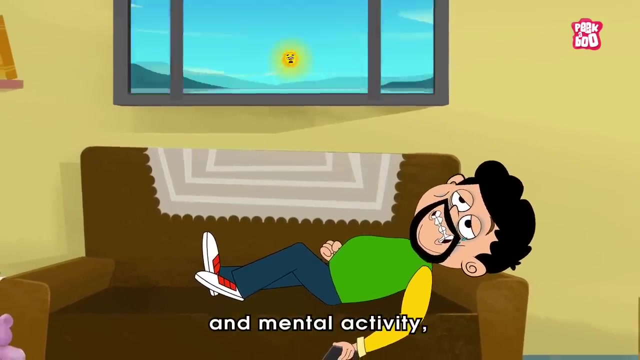 tool that is transforming our lives. but, as they say, with great power comes great responsibility. so it's vital to use ai systems responsibly and not become too dependent on them, as it can make us more reliant on technology and less self-sufficient. this could potentially lead to decrease in motivation and a decrease in physical and mental activity, which would directly